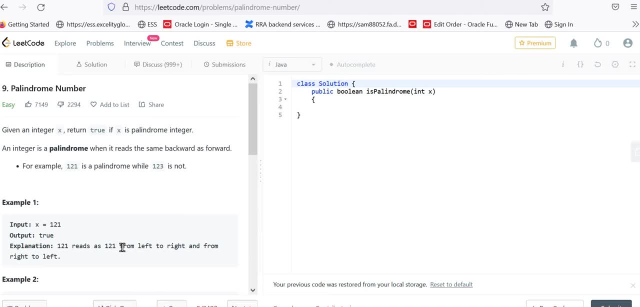 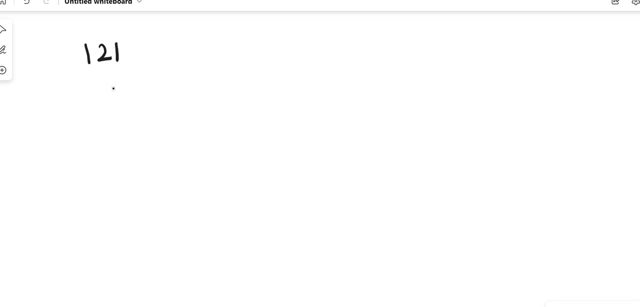 we need to return false. So let's understand the approach, how we are going to reverse the number. So let's take the same number, that is, 121.. Now we have to reverse this number. So how we are going to reverse this number: First we need to extract the last digit, then next digit and then next digit. 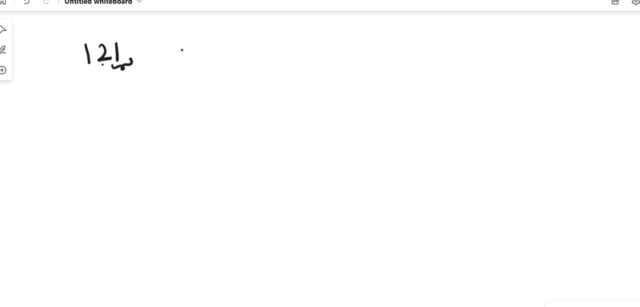 up to the first digit of the number and then we need to store the reverse in some other variable, let's say REV. So how do we form a number If I have to write 121? how can we write this? So if I take the first digit, 1 and then we have to write 121.. So if I take the first digit, 1, and then we 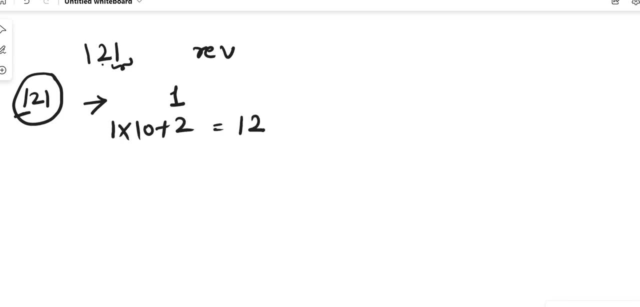 say 0 into 10 plus 2, which would be equals to 12, then 12 into 10 plus next digit, 1, that would be equals to 121.. Right? So if I say here 0 into 10 plus 1, that would be equals to 1. 1 into 10 plus 2. 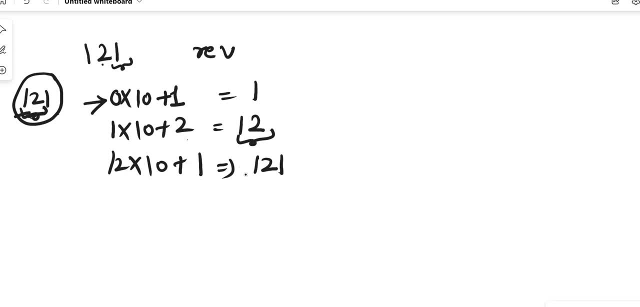 12, then 12 into 10 plus 1, that would be equals to 121.. So can we form a formula from here: If I take any number, for example reverse, if I take reverse as 0. So can I say reverse into 10 plus digit right In the first iteration it would be last digit, then next up to so on. So 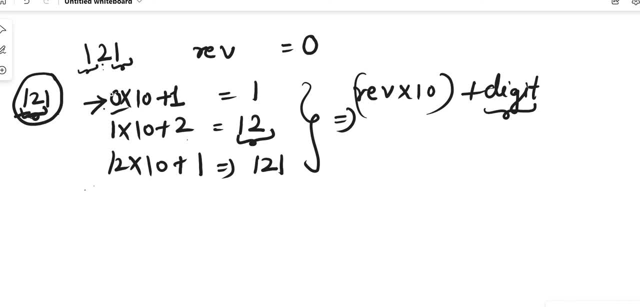 in this case we are taking digits from the starting, but when we are reversing the number we need to take the digit from the last right. So let's say we have a number 121.. So what we are going to do: first we need to extract the digit right last digit and then we have to find 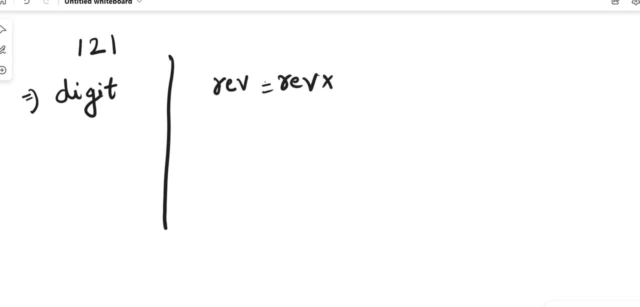 the reverse, which would be equals to reverse into 10 plus digit. This will give us the reverse of the number. For example, in the first iteration. if I have to extract this last digit, what can we do? Can we do 121 mod 10, that means number mod 10.. It will give us always the last digit, So that 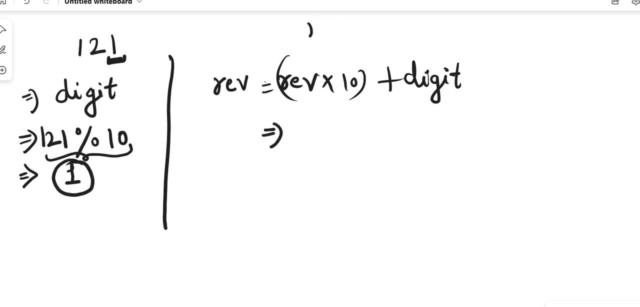 means it will give us 1.. So now in this case? so first we are going to initialize REV as 0. So it will be 0 into 10.. 10 plus 1, that is equals to 1.. So that means we have found our last digit. and then so for. 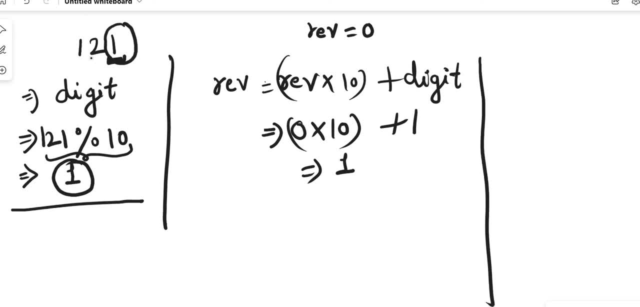 finding the next digit. what do we need to do? Number should be 12, right? Then only we can say 12 mod 10, 2. So to make the number as 12 we need to divide this number by 10. So that would. 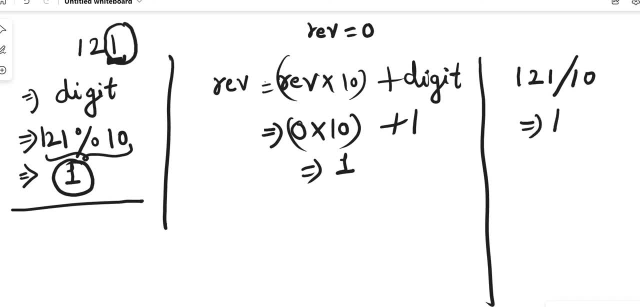 be 121 divide by 10, which would be equals to 12.. Then again in the next iteration: now the number is 12.. So 12 mod 10.. 10, it would be equals to 2.. We have found our next digit. that means this one. So now REV is equals. 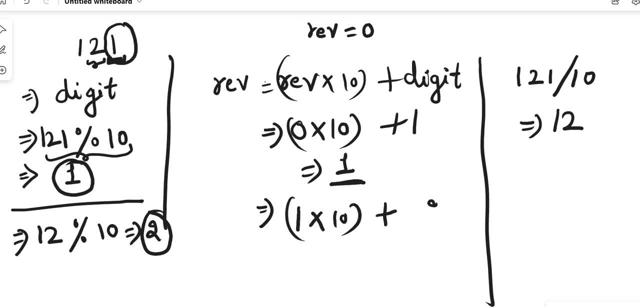 to 1.. So 1 into 10 plus digit in this case is 2, that is 10 plus 2, that is 12.. So now the reverse number is 12, and here we need to do 12 divide by 10, which would be equals to 1.. So now the number. 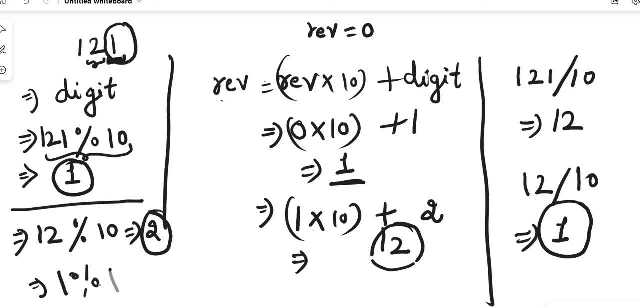 remains as 1.. So that means 1 mod 10, that is equal to 1.. So what would be our next digit? So this is REV. in this case, Reverse is 12 into 10 plus digit is 1, which would be equals to 121.. So that: 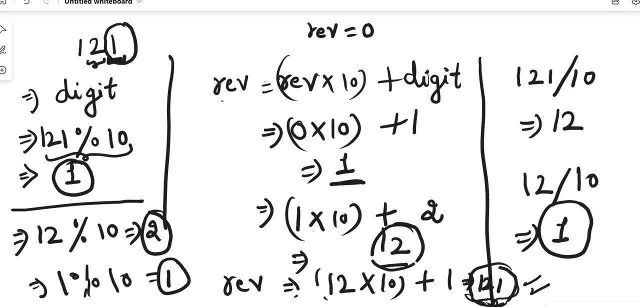 means we have found our reverse number, that is, 121.. Once we found our reverse number, we can just put the checking condition whether this particular number is equal to reverse of the number. Then we need to return true, otherwise we need to return false. So let's write the solution for it, So we 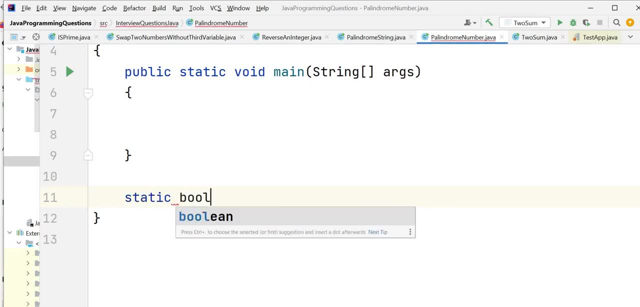 need to write a method which will check whether the particular number is palindrome or not, Since we need to return true. so this method should be of type: Boolean is palindrome and it will take the number as the input And then, since we are going to do the operations on this particular 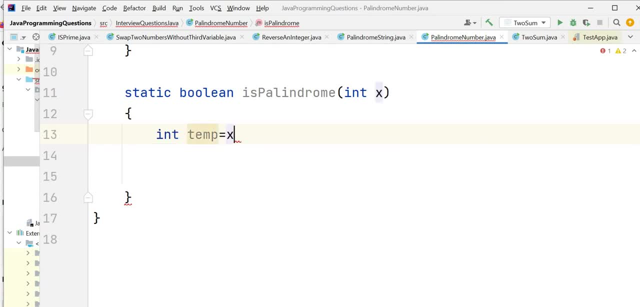 number. let's assign this number to some temporary variable. int. temp is equals to x. Now what was the first step? We need to extract the digit, and then let's initialize REV as 0, and then we can write our loop While this number is greater than 0. first we need to extract the digit. 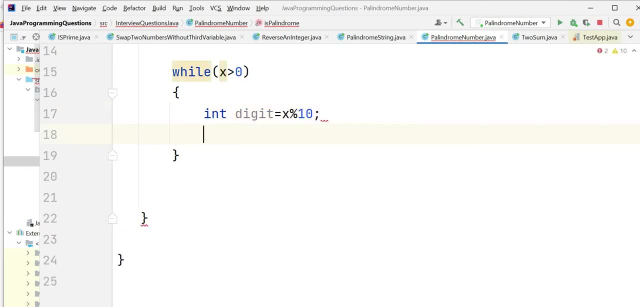 So it would be: int digit is equals to x mod 10.. So it will give us the last digit. and then we need to store the reverse in the reverse variable. So it would be: REV is equals to REV into 10 plus digit, And then, at last, we are going to divide x by 10.. So these were the three steps. First we need: